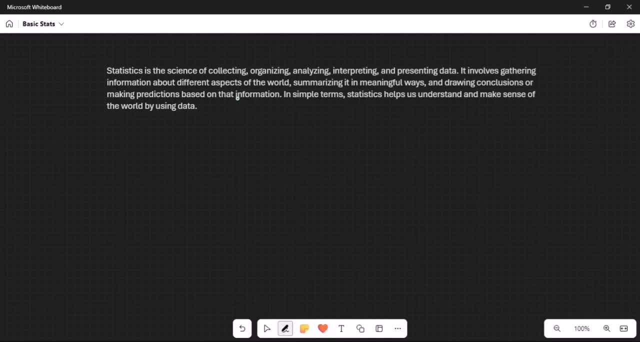 Let's talk about basic statistics today. The most simple definition of statistics that I was able to figure out is this: It might look lengthy, but this is honestly the most simple definition of statistics that I was able to find out on the internet. So here's what it is. Statistics is the science of collecting, organizing, analyzing, interpreting and presenting data. It involves gathering information about different aspects of the world, summarizing it in meaningful ways and drawing conclusions or making predictions based on that information. In simple terms, statistics helps us understand and make sense of the world by using data. 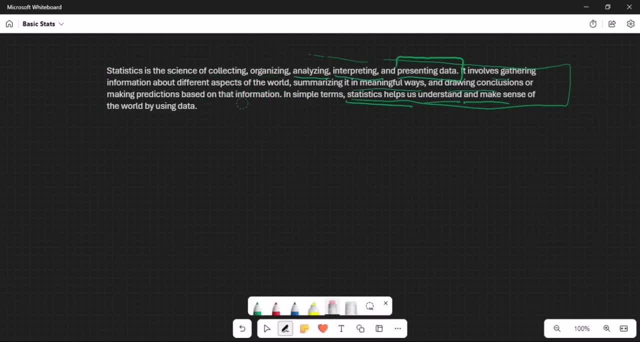 So I would just want you to remember this as the most crucial part of this definition. It helps us make sense of the world by using data. It is a very simple way to organize data, present it and understand it, and then make predictions based on that data. 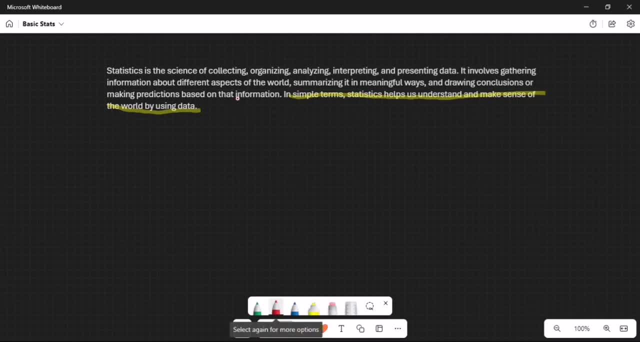 Now here are some basic terminologies that we should talk about before we get into the main topic, and how do we use statistics to interpret, organize, analyze and present data and make sense of the world by using data. But before that again, what is data? 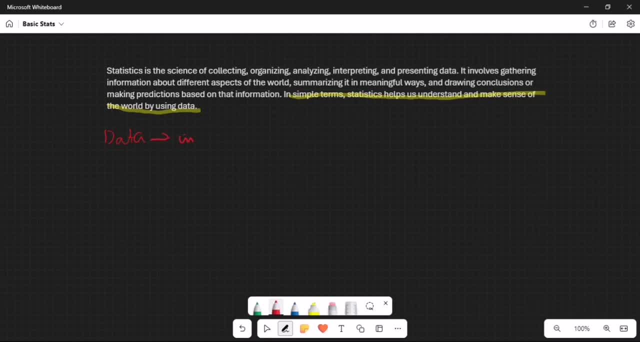 Information From any statistical investigation. Okay now, data can be of one type, which is raw data, which is unclassified or ungrouped data, and it is very difficult to get any meaningful conclusion from it. That sort of data is obtained from surveys, interviews or questionnaires. 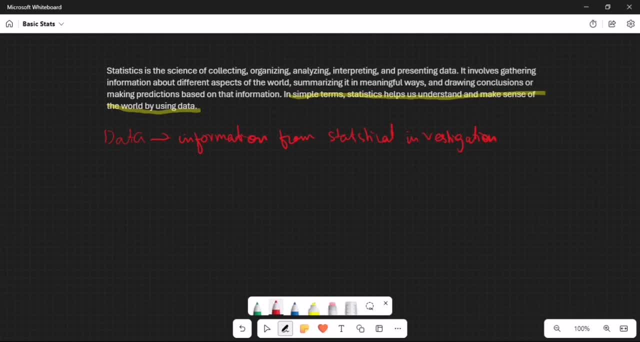 And these sources are also referred to as primary sources of data. after classifying and organizing raw or ungrouped data, we can get useful information through grouped or classified data. Newspapers, reports and articles that are straight data are called secondary sources of data because these data come from primary sources, which are surveys, interviews, questionnaires or whatever. 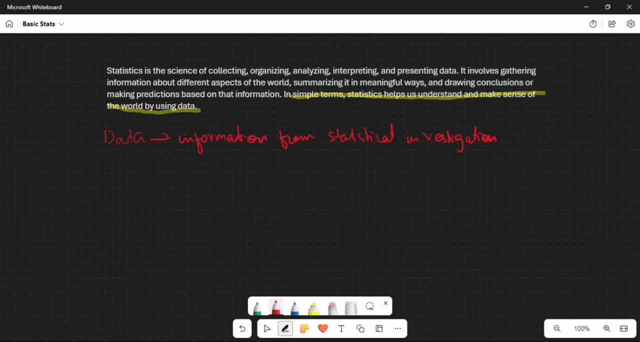 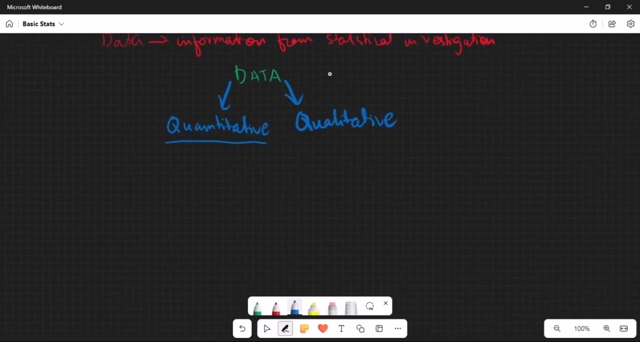 Let's look at some examples Now. data can be divided into two main categories: Number one, quantitative, number two qualitative. Now, as the name suggests, quantitative data is data that is all about quantity, it deals with numbers, and quantitative data is about qualities like color, material, what an object. 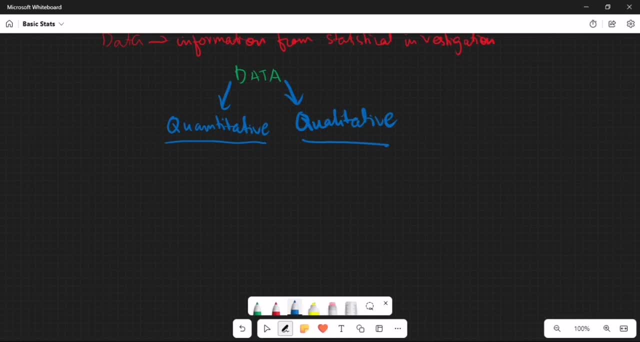 is made of, Is it plastic, steel or any quality? So I think the meaning of quantitative and qualitative data is pretty obvious by the words themselves. Moving on, here are some examples again: Data on gender, blood group, eyebrow, color grades, roll numbers are qualitative data. 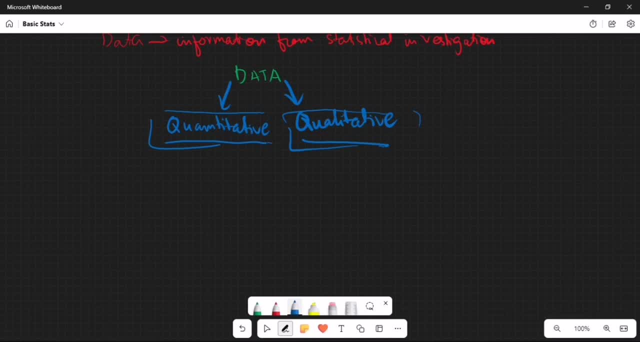 Data on height, weight, salary, pH, values of solutions, annual profits of company, marks, of students in a subject. Now, observations and qualitative data are purely attributes without any numerical significance, but these may or may not possess ranking or ordering like ascending or descending order. 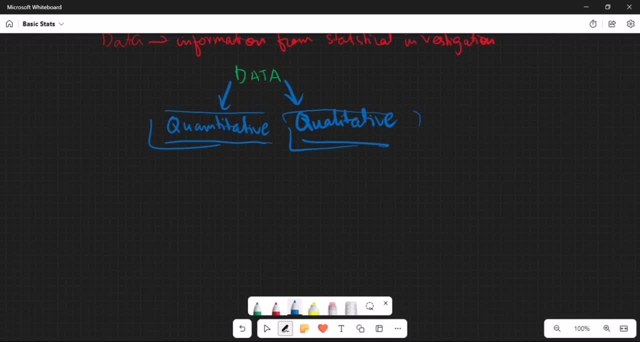 Now there are two types of quantitative data again, one that does not possess ordering- as I said before, it may or may not possess ordering- but one that possesses ordering is called nominal And the other one is called ordinal. Let's talk about the ordering thing in qualitative data later on. 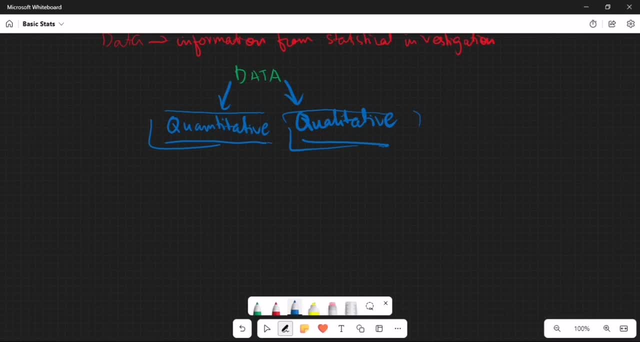 Moving on observations in quantitative data. now these are numbers with numerical significance, unlike qualitative data, and they have ordering, for obvious reasons, So quantitative data is always ordinal. Now these numbers can be integers only or also indexed, So quantitative data is always ordinal. 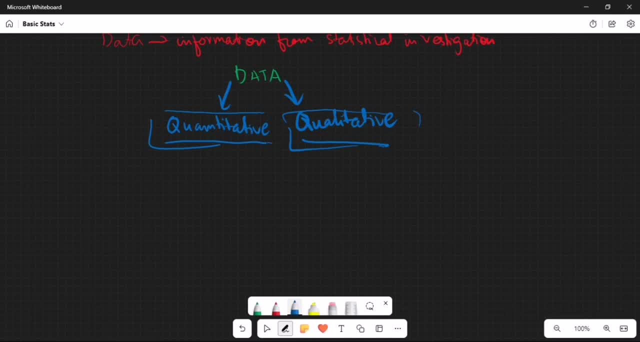 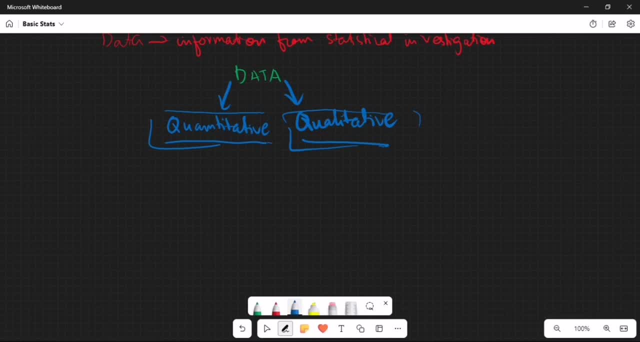 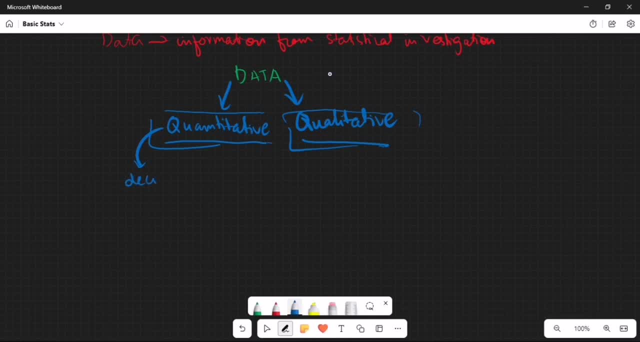 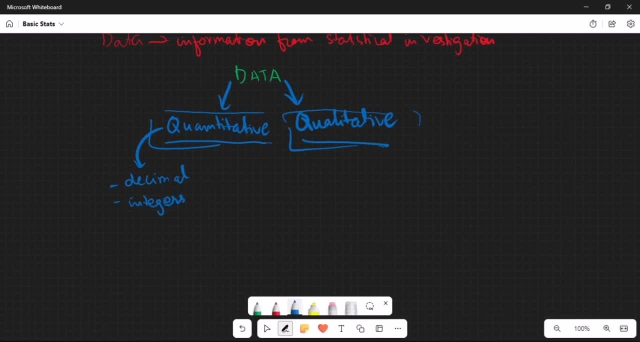 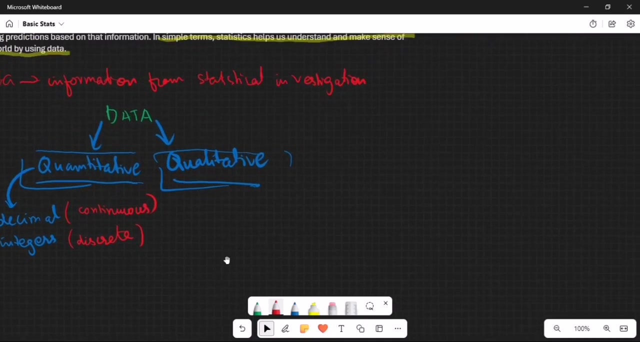 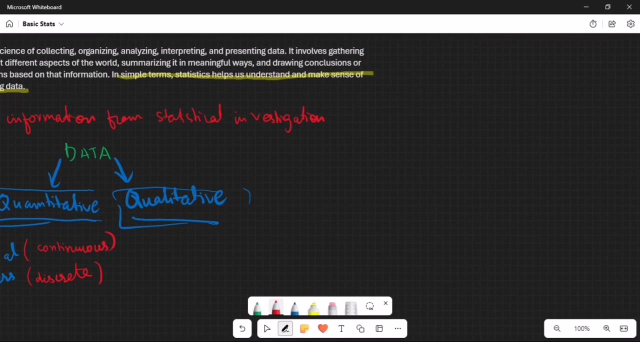 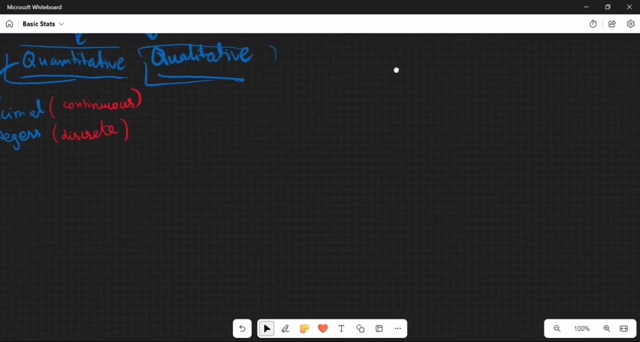 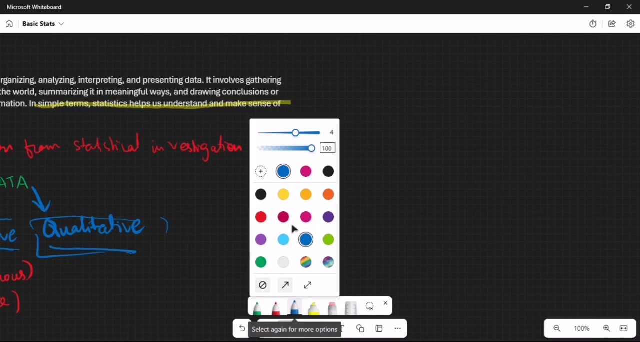 Now these numbers can be integers only or also indexed, and the one that has decimal numbers is called continuous and the one with integers is called discrete. okay, moving on, the next important term in basic steps is frequency distribution. you, okay. in order to get meaningful data from statistics, we need to classify into: 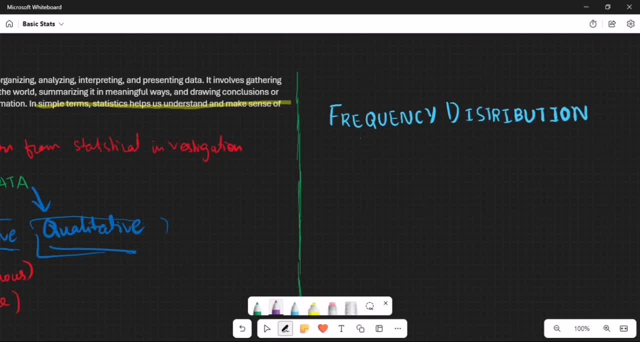 smaller classes or quarters. now, as we already discussed, quantitative data can be of two types: discrete or continuous, based on the type of number it has. so the discrete classes, the data up, oh yeah, the data. the classes that have discrete quantitative data comprise of a single number slash attribute, whereas continuous classes, 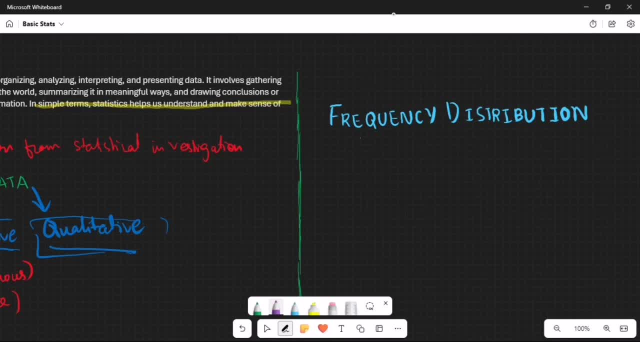 contain a range of numbers for, like, a discrete class would simply say, okay, fifty-nine, but then a continuous class would say sixty-nine to maybe like eighty-nine. so it gives you a range. this is what continuous data would look like and this is what discrete data would look like. okay, now moving on the 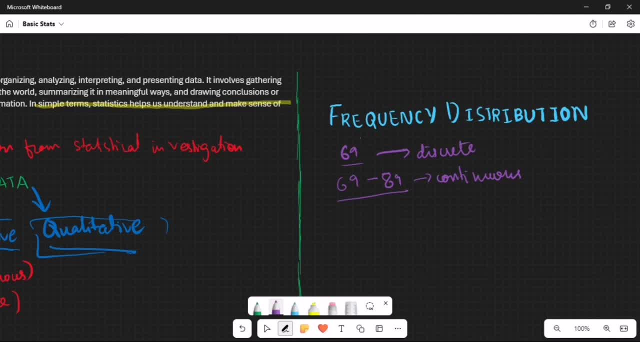 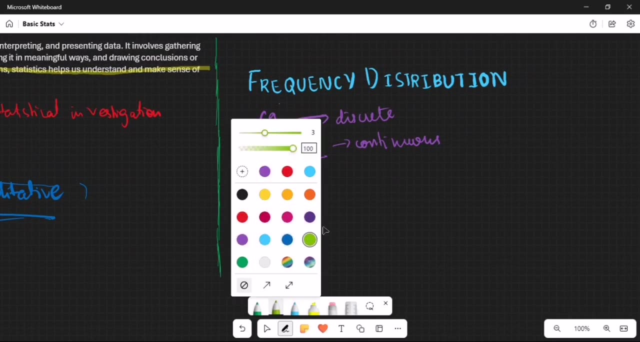 number of observations falling in a particular class is called its frequency. so basically, whenever you're forming a table of data in statistics, the first column- I guess for now, as we are on the basics, is all about class. so, for example, I've got any data of various blood groups. let's say a positive. in fact, let's have 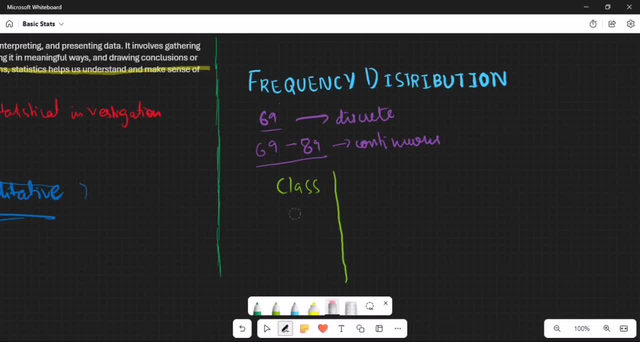 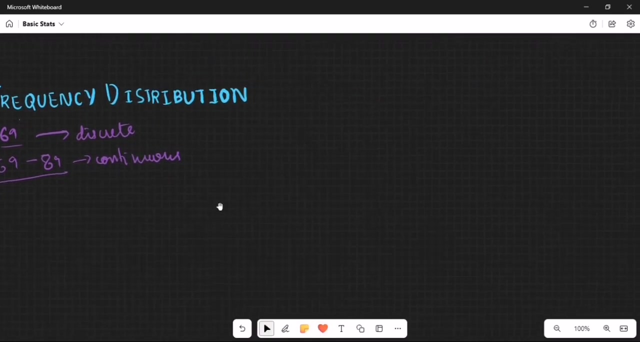 some separate space for the question so that we understand it in a better way. okay, so what we learn in statistics is that theaque, all the elements, both of them are all the same, so you can get any data in仯 and you know, so you can find any value from the display fluid. here's the value of the hierarchy. 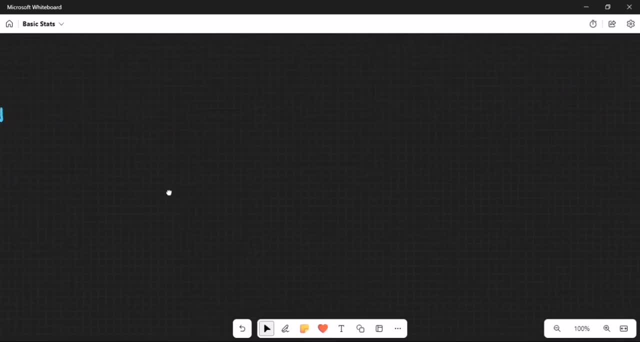 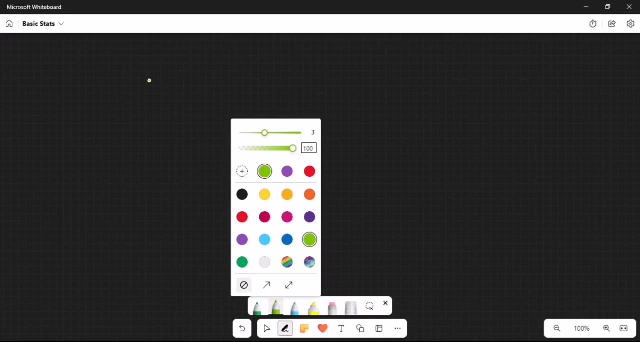 and type those in the randomness to the reference elements, all those fields that are related to this. the íl, when you want an estimate of the quantity, at which we have three items, is the variable of volume. okay, so we will justiven the variable over here. let's construct a table for this data. 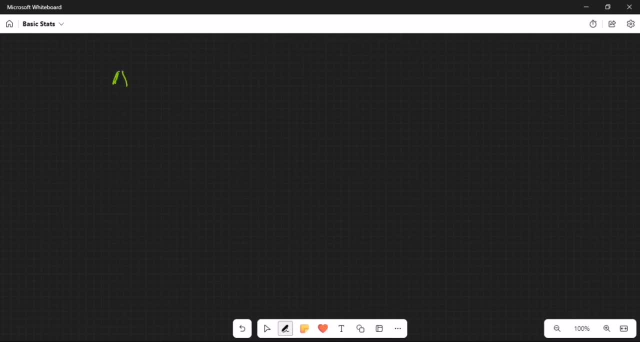 let's say, we have some data, like we have various blood groups and data about it, and we're supposed to construct a table for it, a frequency distribution table, to get meaningful information out of this data. so let's do it. okay, this is so in the question we're 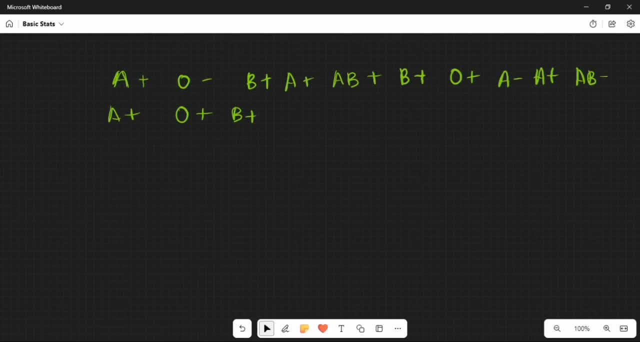 supposed to construct group frequency table of the blood groups of these students of a class. okay, so we're constructing a frequency table. oh, there are two ways to do it: number one, frequency table with discrete classes and number two, frequency table with continuous classes. for now we're talking. 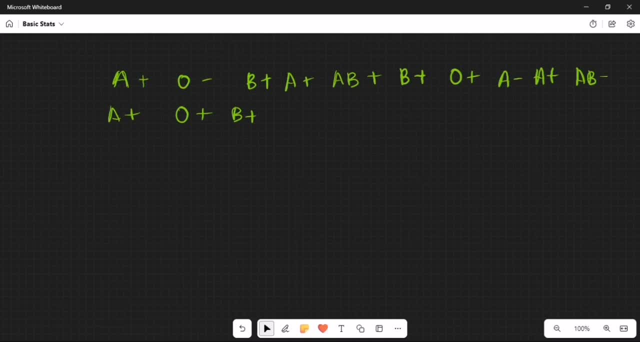 about frequency table with discrete classes. that is not helpful. have a range, so the street classes are the classes with only a single number slash attribute to include similar observations. we use it when few observations repeat more than a number of times in the data. so frequency table of discrete classes is also. 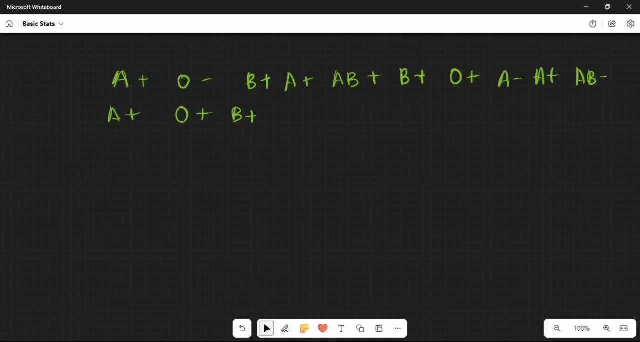 referred to as discrete frequency table. so whenever you're given a data set like this, this is called a data set, a set of data. so whenever you're given a given a data set number, one thing that you're supposed to do is identify observations as classes. so these, what are these? what? 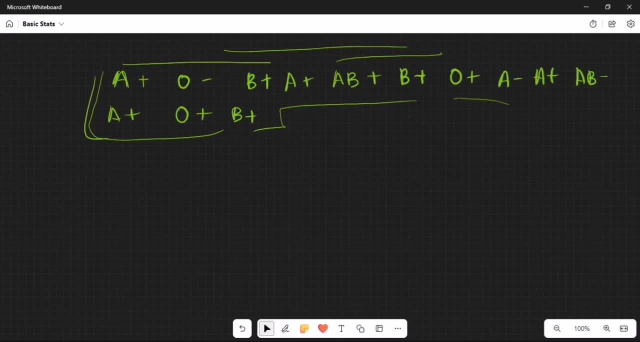 this data. are you doing Den? I was a student here last semester because I wasáveis have dumbass. okay, I know I theater usually. okay, I know I did was very day super important part of this strategy, king, that makes you wow. okay, even your actions. now you're entering a fundamental 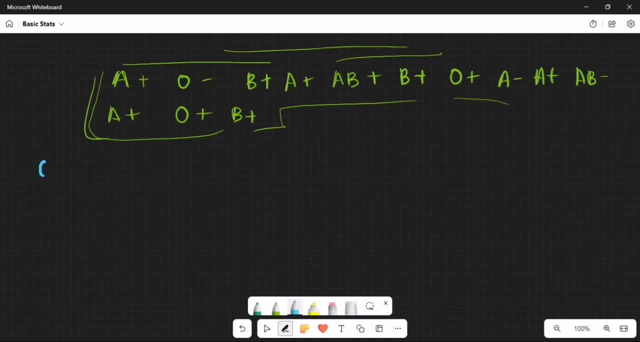 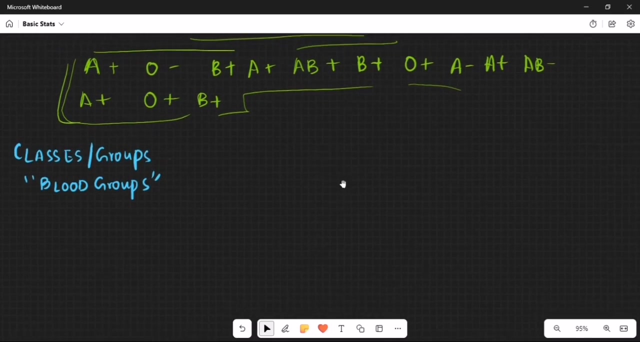 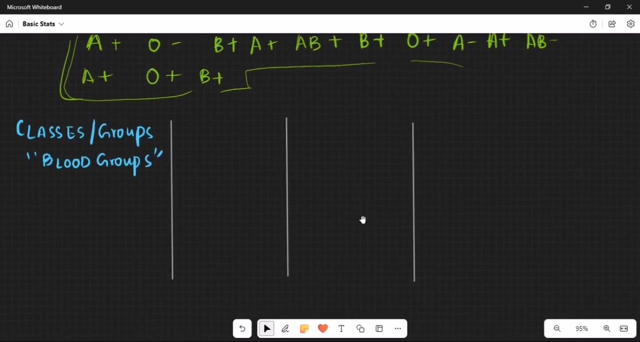 it classes, slash groups, and in this case, what are the class of groups? blood groups. let's make it meaning clean so that we again get meaningful, actually get meaningfully out of it. ok, so I think this makes it better. moving on, let's finally make the group frequency table for this discrete data.